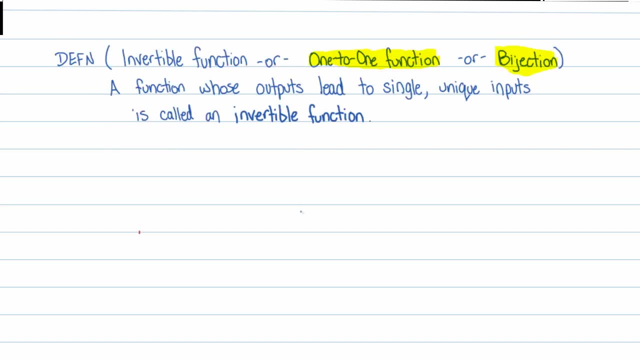 and all that fun stuff. At the end of the last lecture, the conceptual lecture, I had mentioned the definition of an invertible function, a function whose outputs lead to single, unique inputs. It's called an invertible function. I just want to mention that here because we're about to. 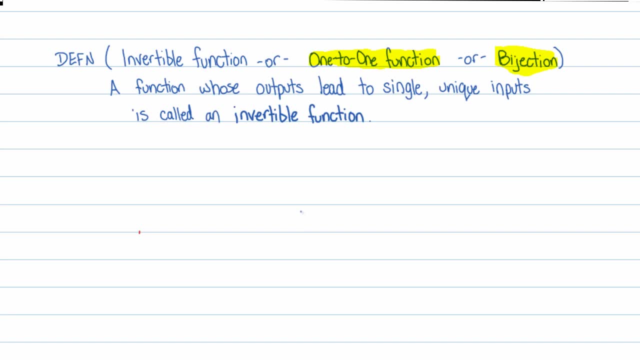 use that language in another definition, and that definition is for function notation. Let f be an invertible function, which we just said is just a function whose outputs come from unique or single inputs. Then we denote the inverse function that is related to f by this notation. 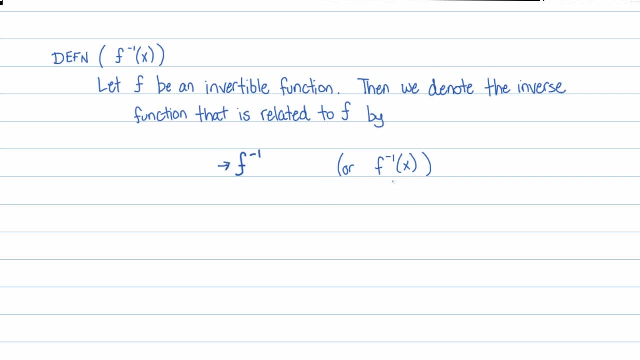 Or sometimes, more often, actually by this notation. I think a lot of students get confused about this. f is the name of the function here, f of x is the value of the function evaluated at x. So its inverse has a name, f, and I'm not going to say raise to the negative one Instead. 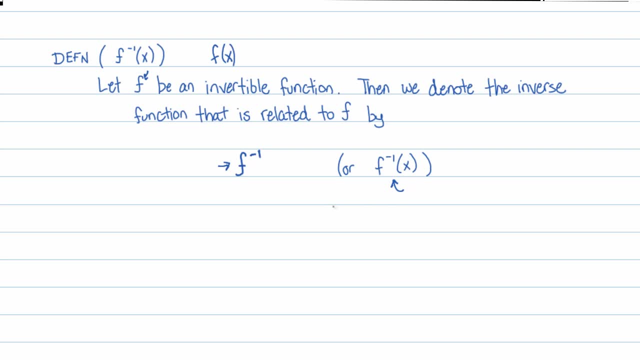 you say f inverse And then that value is that function? is the inverse function value evaluated at x is f inverse of x. A couple of things I need to warn you about here. F inverse is not equal to 1 over f. It's a such an unfortunate notation that they chose. 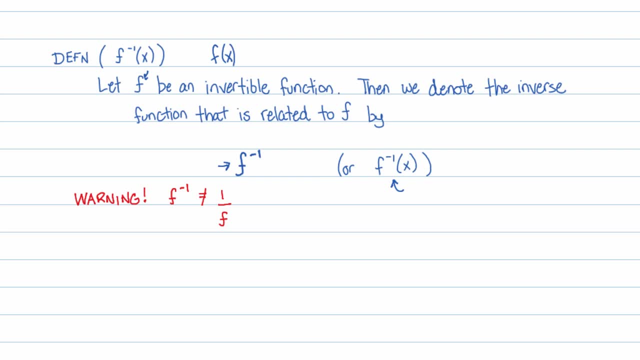 or whoever chose it for inverse function notation. They should have gone with something absolutely different, because we have negative exponents And so we're so used to seeing a negative exponent saying: rip off the negative and drop that downstairs. But when you're talking about a function f, that's a function name, and when I see a negative 1 as a superscript, I know they mean the inverse of f. not necessarily 1 over f, it's the inverse of f. whatever machine undoes f. 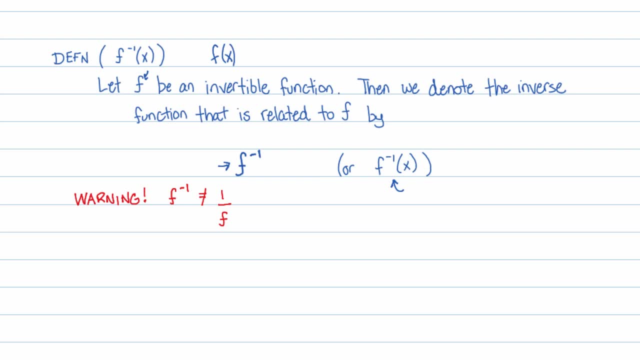 Extremely unfortunate notation and I would love if somebody would come in and actually change that notation. Personally, I would love to see something like arc f or something like that. The reason why I choose arc f is because in trigonometry you deal with inverse functions and they always title their inverse functions or pre-title them with an arc. 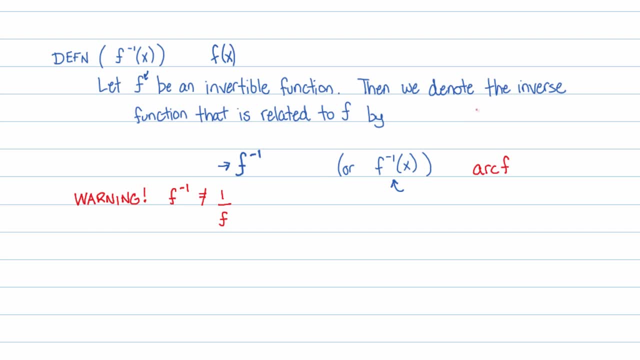 So it would be an arc cosine or an arc sine or something like that. Not that you need to know that, but it's a better notation than this. This sucks Anyhow. another thing that is from poor notation: here I will often like to write f inverse of y. 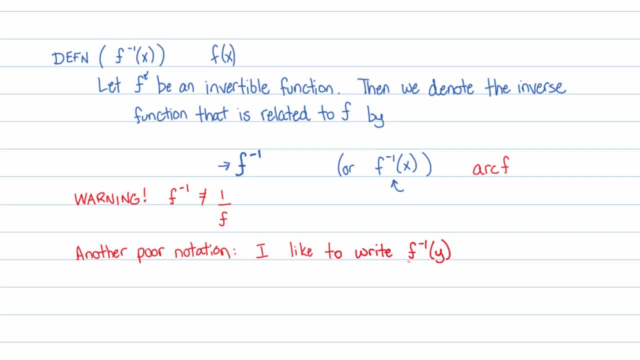 Now, we're so new to this you probably don't know or understand why I choose to write it that way. But let me just tell you: if a function is equal to f of x, in other words, if my function name is f of x, so in other words, y is equal to f of x. 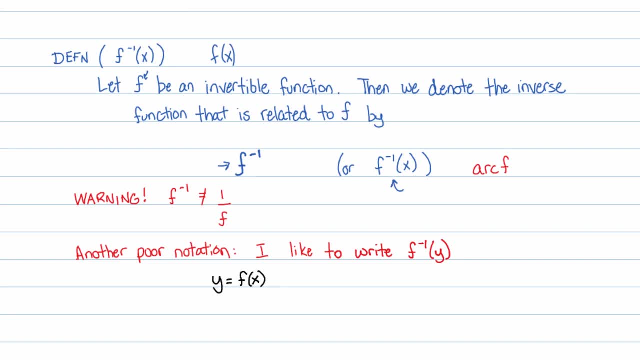 that means for my function I'm plugging in x values and I'm getting it And I'm getting out y values, correct? So remember from our previous conversation with the conceptual conversation with inverse functions, the inputs for an inverse, what goes inside these parentheses, should be the outputs of our original function. 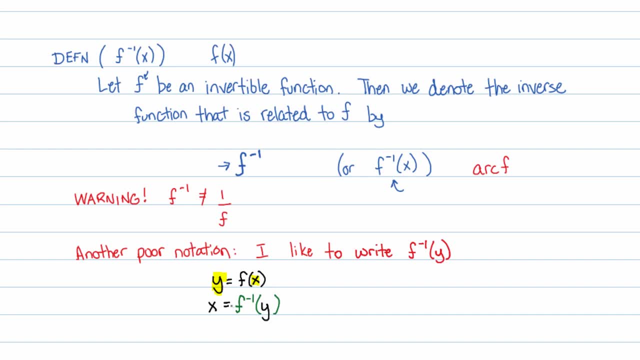 This is technically absolutely 100% correct, But the problem is that every single textbook that I've ever seen writes this as y equals f, inverse of x. In other words, they use this notation And I think it's a very poor notation because it's extremely confusing. 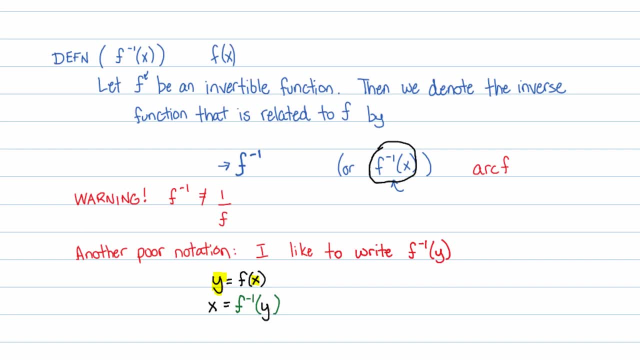 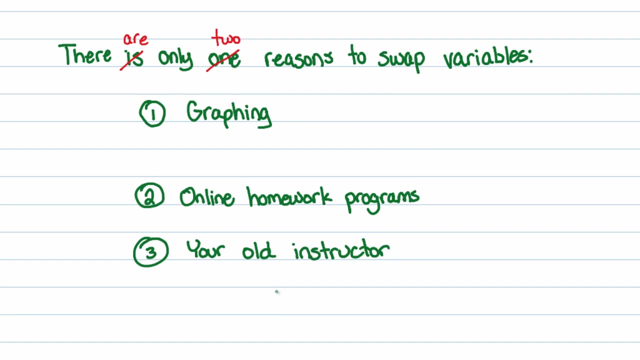 And in real world problems, you would never, never, never, never, never, never swap those variables. But every single textbook teaches you to swap variables. There's only one reason to swap variables. Nope, There are only two reasons to swap variables. 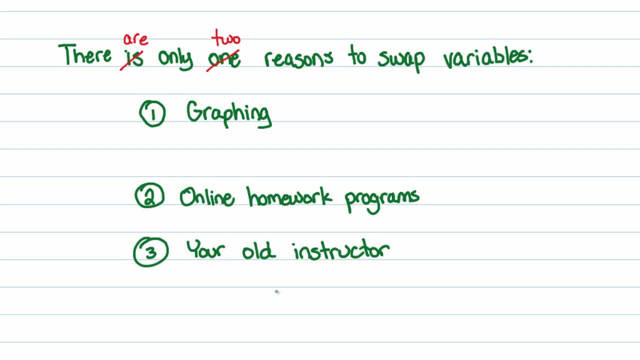 One reason is for graphing. That's actually the only real reason. That's the real reason right there for swapping variables. If you're going to have to graph an inverse function, you have to swap variables. That is very true, Okay. 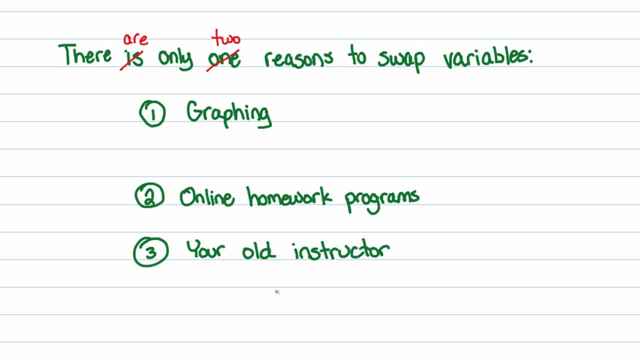 Fine, I'm all right with that. Okay. The second reason, which is not a real reason, but it's a- The reason that most students have to contend with these days is for online homework programs or online homework systems. They all swap variables. 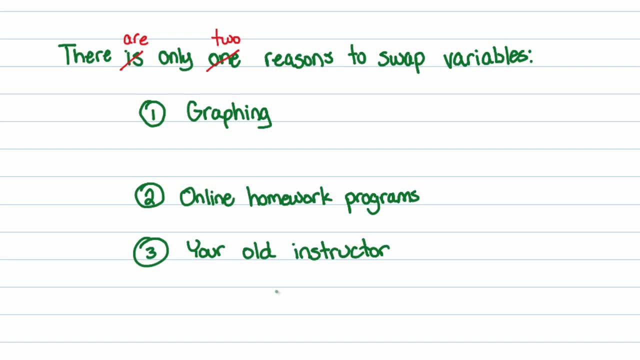 And every textbook does as well. So, because if you're using an online homework system, it's going to require you to swap variables at some point if you find an inverse. And finally, your old instructor- not your old, your previous, I mean your old school instructor. 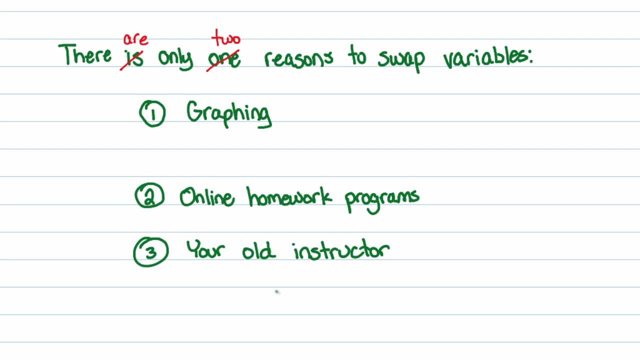 your instructor, who doesn't know why they do something, they just do it. You should ask your instructor actually Why, Besides graphing, why do I swap variables? And they'll probably have no answer for you. If they do come back, tell me. 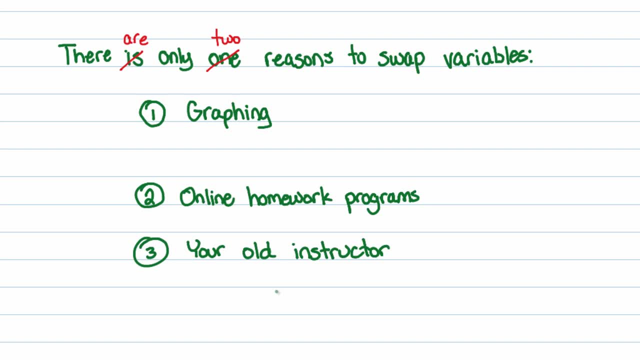 And I'll give you. I'll probably argue it with you, But that's absolutely fine. I think that these last two points are not valid enough to swap variables. This one right here, pretty valid to swap variables if I'm going to graph. 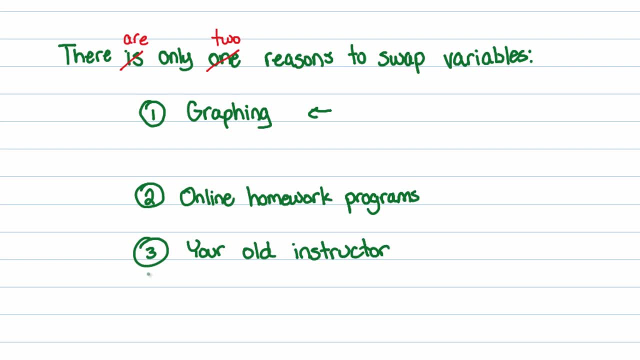 Now all of this makes very little sense to you, So I'm going to come back to this in probably another lecture here, when I go to graphing these things and finding And equations or function- Yeah, basically equations for inverses, But for now, let's go ahead and learn to use function notation. inverse function notation. 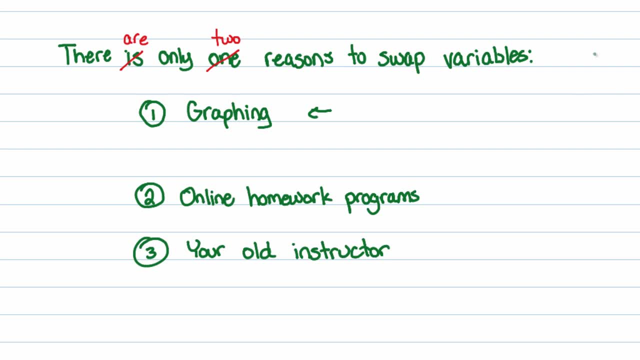 By the way, you're probably wondering why I say there are only two reasons to swap variables and there are actually three reasons here. It's just because of an old joke. There are three kinds of mathematicians: those who can count and those who can't. 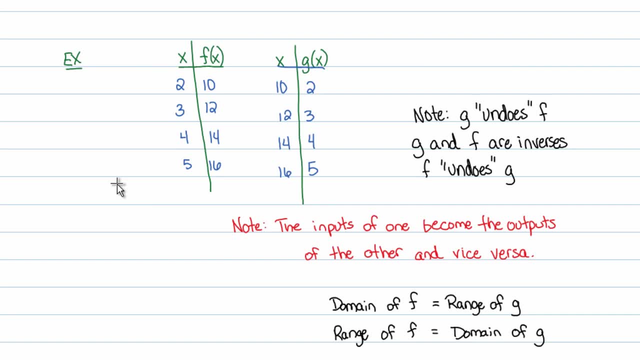 Ha ha. Now talk about function notation. Now talk about function notation here and how we're going to use it. I'm going to go back to some of the examples we had in the conceptual lecture. Here we had a function name, f. 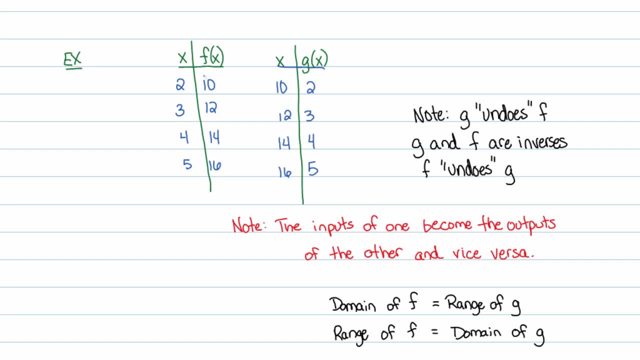 So when you plug 2 into f, f of 2 turned into 10.. When you plug 3 into f, f of 3 was 12, and so on and so forth. So all these imply that f of 2 is equal to 10 and f of 3 is equal to 12.. 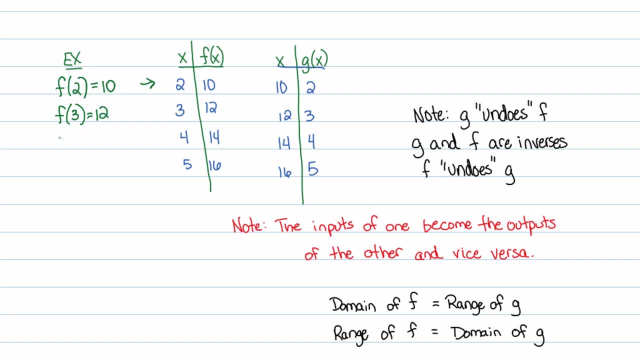 And so on and so forth. But now that we know that these two are inverses from the conceptual lecture- remember g undid f. g and f are inverses. The inputs of one become the outputs of the other, and vice versa. In other words, the domain of f is the range of g and the range of f is the domain of g. 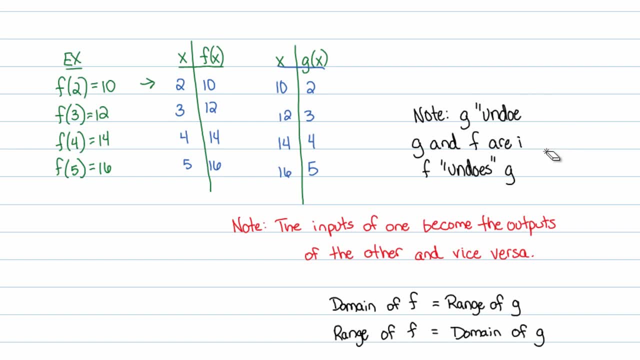 Well, because of that, I now know that another name for g, and probably a more proper name for g, is f inverse And the unfortunate notation f inverse of x, and I'll show you as an example why this is a bad notation in a moment. 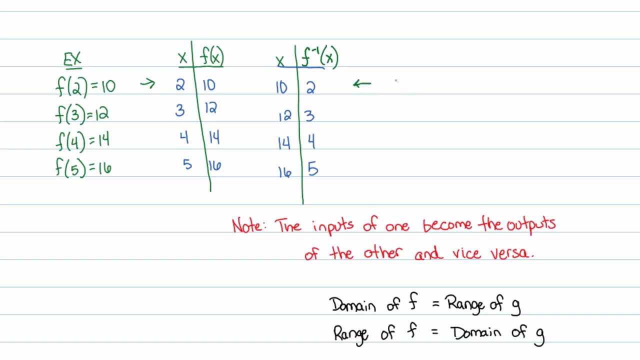 Let's go ahead and just say what this implies. This implies that f inverse of 10 is equal to 2. And f inverse of 12 is equal to 3.. And f inverse of 14 is 4, and so on and so forth. 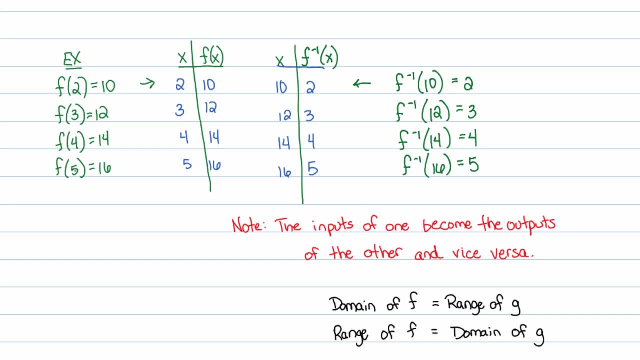 Alright. notice that the inputs for f lead to outputs and those outputs are now the inputs for the inverse of f. Now again, I hate, hate, hate, hate, hate, hate this poor notation. But that's not your fault, that's the fault of every mathematician in the world. 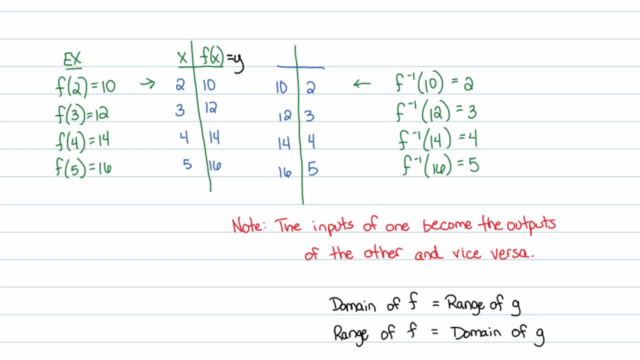 This f of x we always call y. right, The input is x, the outputs are y, So another name for f of x is y. Well, if the inverse takes those outputs as its inputs, oops, that should be an inverse sign. 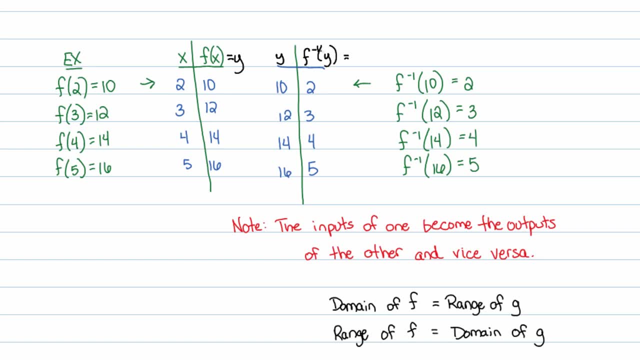 then when I plug in those outputs into the inverse, it should return the original inputs. I like that notation so much better. it just makes sense, right? It's like you just swapped columns. that's really all you're doing. So what a frustrating notation that all mathematics has kind of adopted. 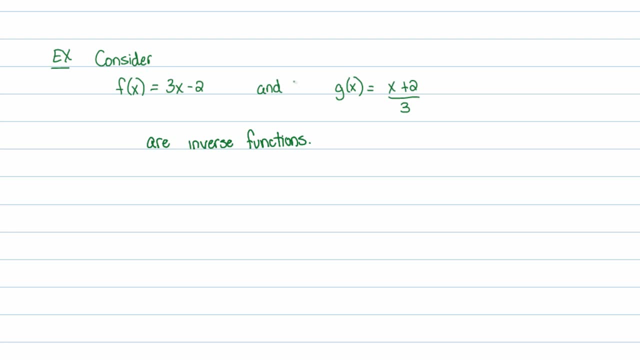 Again. from the previous lecture on the conceptual approach to inverse functions we found out that f and g here were inverse functions, so in reality there's no reason to call that a g. it should actually be f inverse, officially f inverse. 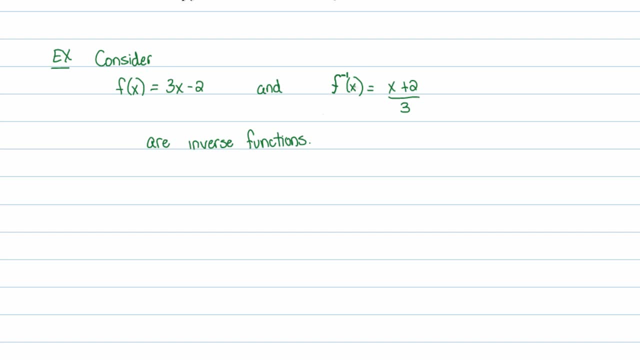 And really, since it doesn't really matter what variable letters I use, I can make this f inverse of happy face if I really wanted to right. It doesn't really matter what variable I use. A lot of people use x because they're just happy with using x's all the time. 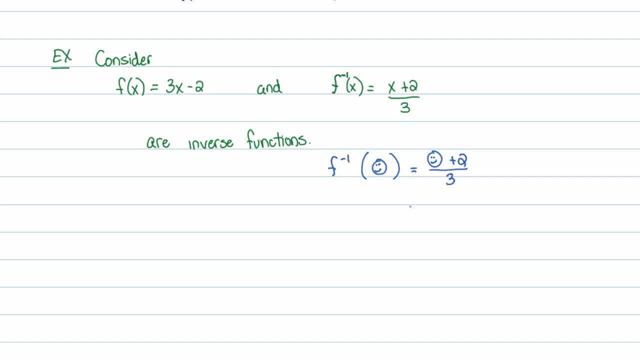 But in reality it doesn't really matter what variable you use. So if it doesn't matter what variable I use, I'm going to do this. f inverse of y is equal to y plus 2 over 3.. Just because it makes sense. to me, this makes absolute sense. 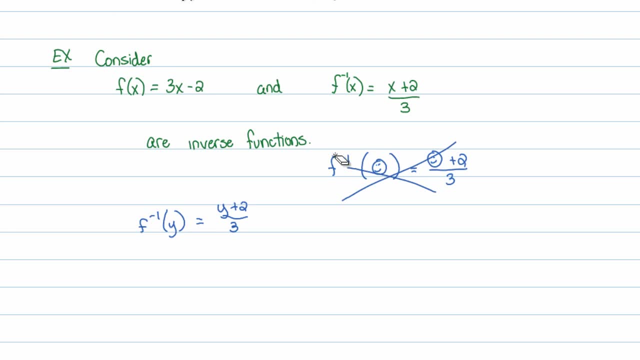 Now let's see why this makes sense in this: not only this case, but all cases. Now let's see why this makes sense in this: not only this case, but all cases. Now let's see why this makes sense in this: not only this case, but all cases. 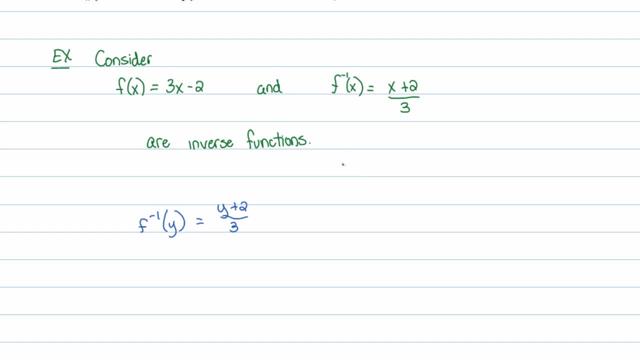 Because let's say, we want to evaluate f at 30. So I plug in: x equals 30, so wherever I see an x here, I replace it with a 30. So this is nothing new. I just evaluated a function. 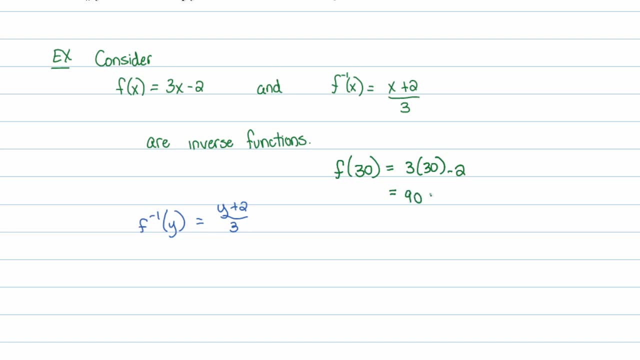 that's three times 30 is 90.. Minus 2, which is 88.. Now remember, This is a y value. This is an output. I plugged in a value of x. I should have gotten out a value of y. 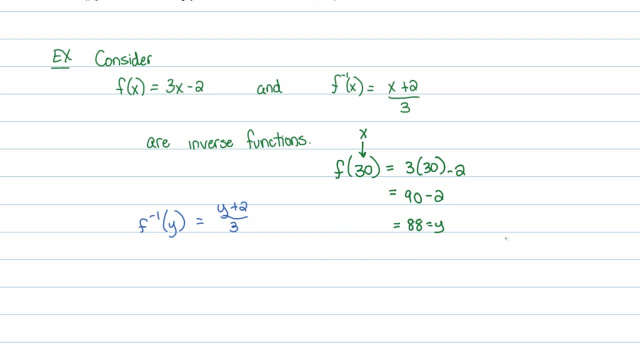 The inverse should take that and return back the original input. So the inverse function which I'm going to say my inputs are the outputs of my regular old function. so the y values, The inverse, I'm going to plug in that output of 88.. 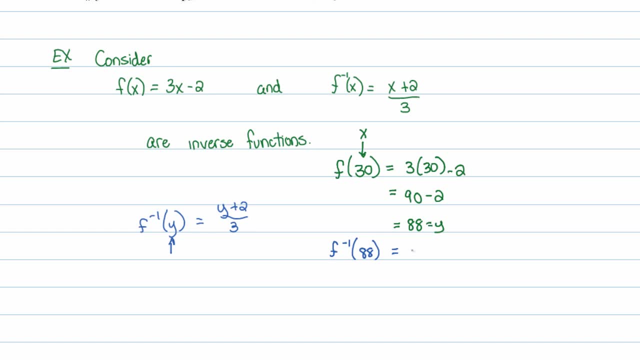 Well, let's see, The inverse is just y plus 2 or 88 plus 2.. Over 3.. 88 plus 2 is 90.. Over 3 is 30. And remember, if you look at this notation f- inverse of y. so we're plugging in y, we'll get out x. 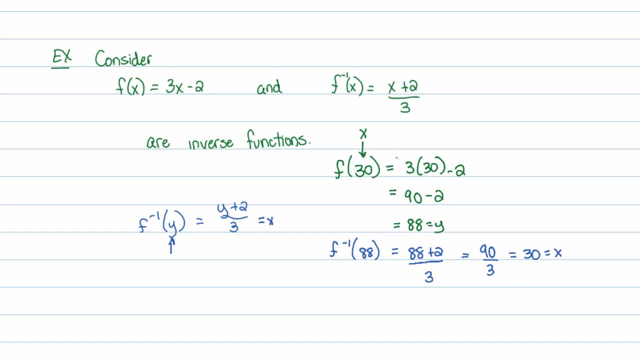 So this should equal x, And it does. Originally we started with x equals 30. It changed into a y equals 88. We plugged in y equals 88 into the inverse. It turned back into x equals 30. But again, 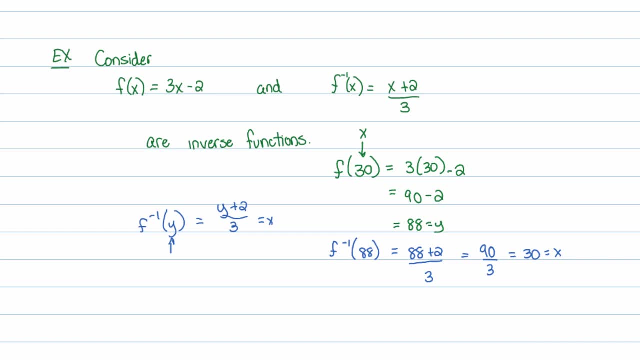 Your textbook will never say. I'm taking a wild stab. If you have a textbook that doesn't say what I'm about to say, then you've got the first textbook that I've ever seen without this notation, But most every textbook I've seen has this.